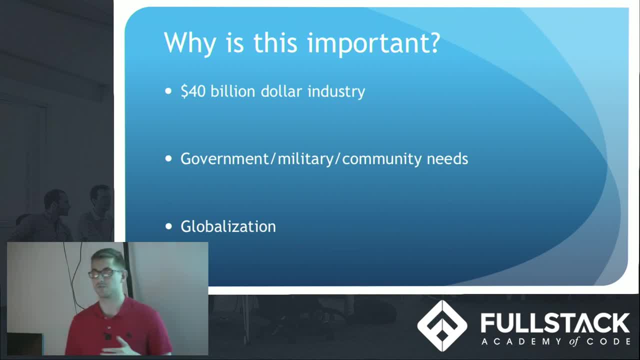 Military, our armed forces who are going overseas. We have to be able to communicate to the locals over there And our community Here in New York. every day, I'm sure you hear a different language that's not English, So it's really important that we're able to communicate with one another. 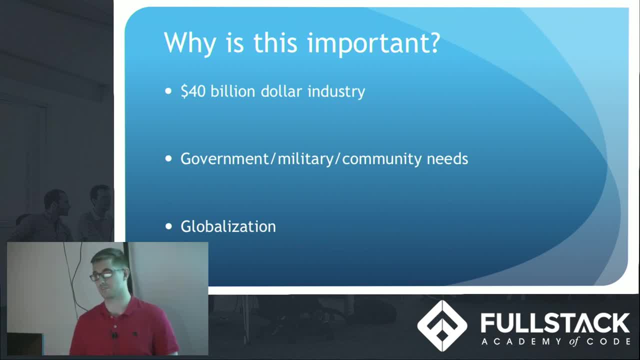 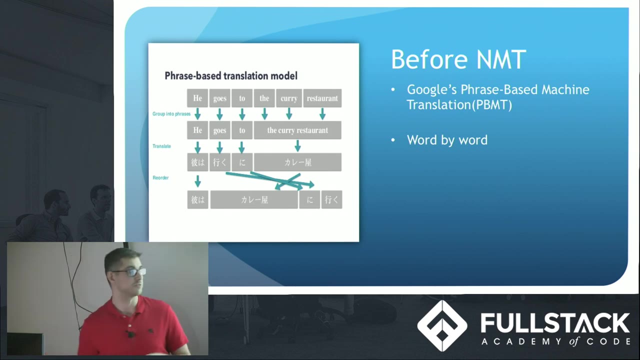 And globalization. If you want to start a business abroad, I don't think you'll be able to just speak in English, especially if you go somewhere in Asia. Before NMT, So before neural machine translation, Google especially used this phrase-based model, which was PBMT. 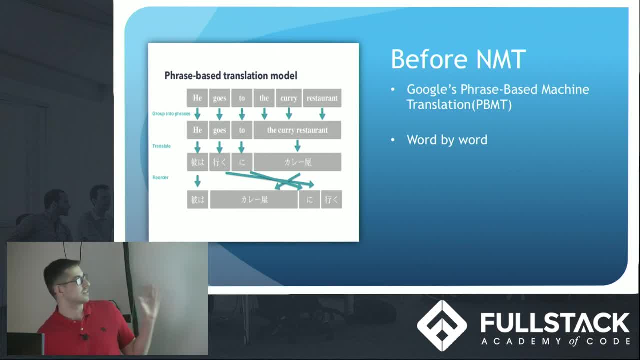 where, as you can see, it's translating this sentence word by word. So he goes to the curry restaurant was translating he to. he goes to goes two to two. The curry restaurant was grouped as a phrase and then translated into Japanese. 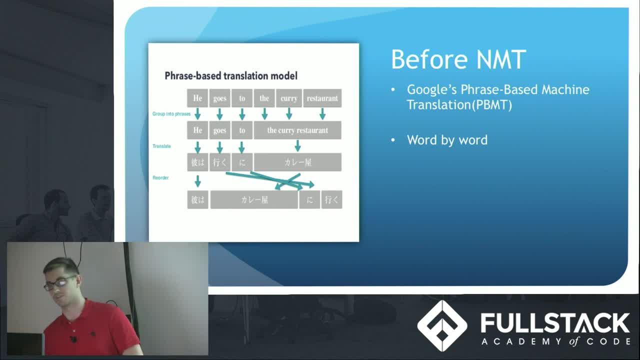 and reordered based on the Japanese grammar structure. You may think that this is fine. I mean, you get a translation. Not any of you, I don't think, can understand the Japanese, but it's a fine translation. But what happens when you get to more complicated sentences is you lose context. 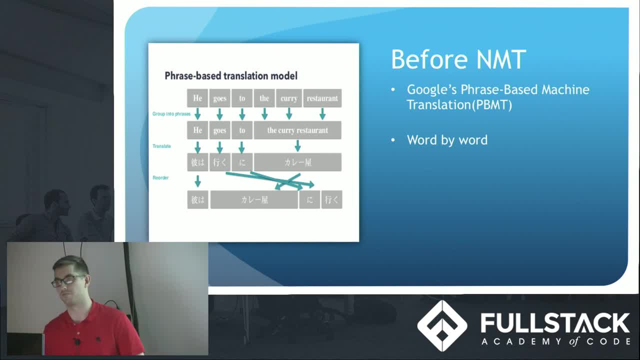 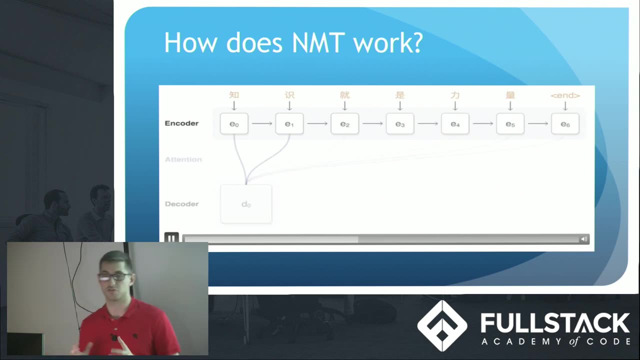 If you don't remember the previous words beforehand, you're going to get an inaccurate or poor translation, And that's where NMT comes in. So NMT is a new approach to machine translation that uses a large neural network to enhance performance. In other words, the computer uses deep learning to build an artificial neural network. 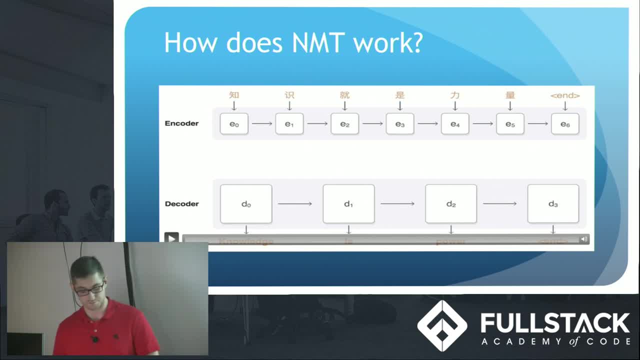 to teach itself how to translate between languages. It uses these neural networks to translate entire sentences without breaking them down into smaller parts. So I'm going to come back to this visual. Let me restart it because I don't think you have to pay attention here. 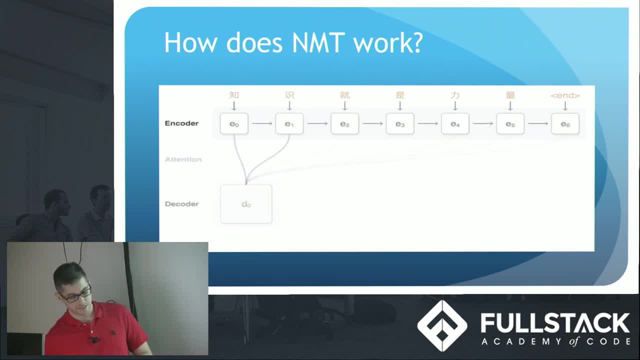 because each Chinese character is being read in this top encoder. Once the entire sentence is read, it is then finally decoded, one word at a time in English, And one more time. you'll see this attention, You'll see this attention here, come up. 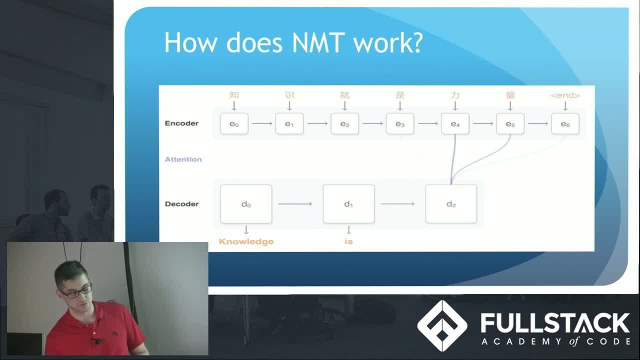 where that is giving a weighted distribution over the encoded Chinese words most relevant to generate that English word. And the important thing about this is it keeps the context of the sentence And, as I mentioned before about this zero-shot translation model, this was one of the coolest things I thought. 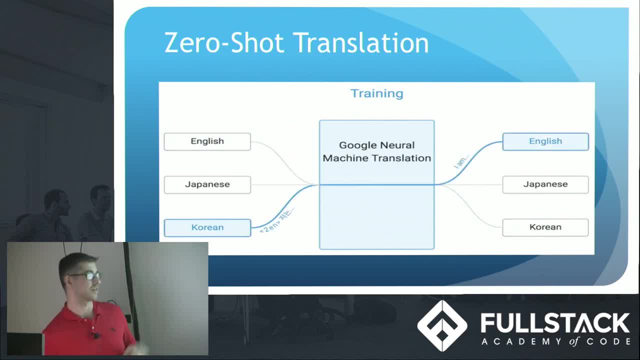 when I was doing my research. So this computer is being trained to translate from English to Korean, Korean to English, English to Japanese and then Japanese to English, And without seeing any training data for Japanese to Korean, it has taught itself how to translate from Japanese to Korean. 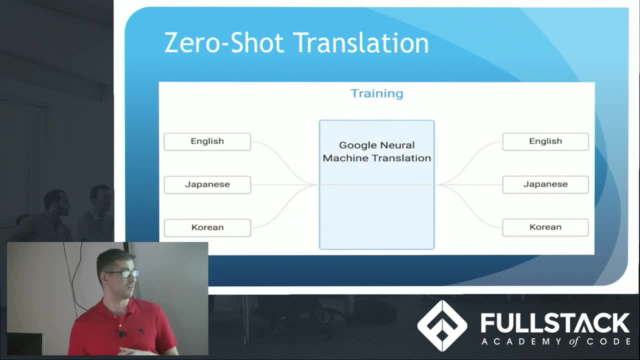 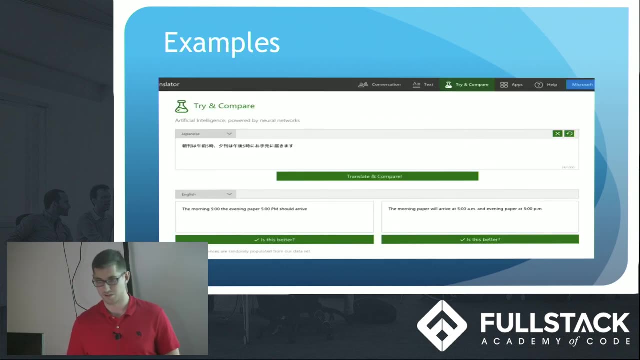 and Korean to Japanese. So I thought that was a fascinating and huge advancement for translation in general. And now I want to move on to some examples, just so you guys can really get an understanding of what's happening here. So I have this Japanese sentence up top: 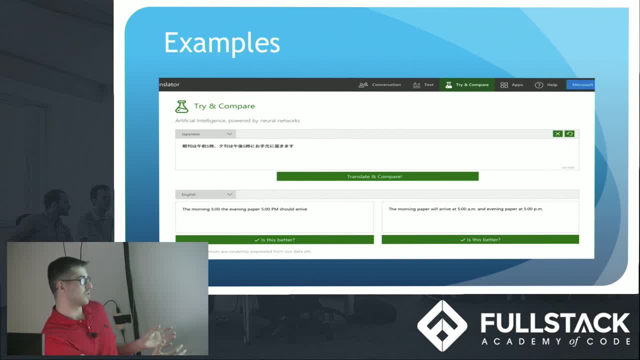 And Microsoft Translator gives you two different translations. One is the old statistical model, or what Google Translate called their phrase-based model. The other is the new neural model. So this Japanese sentence up top translates down below: The morning 5 o'clock. the evening paper 5 pm should arrive. 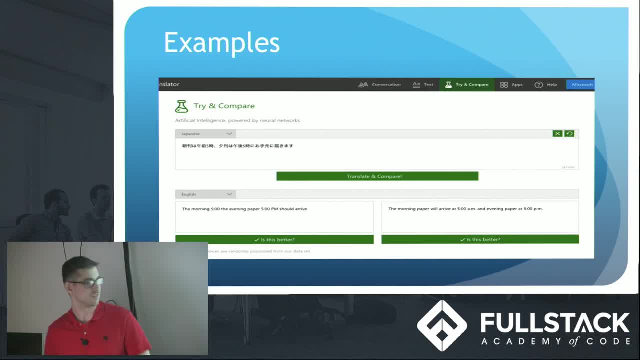 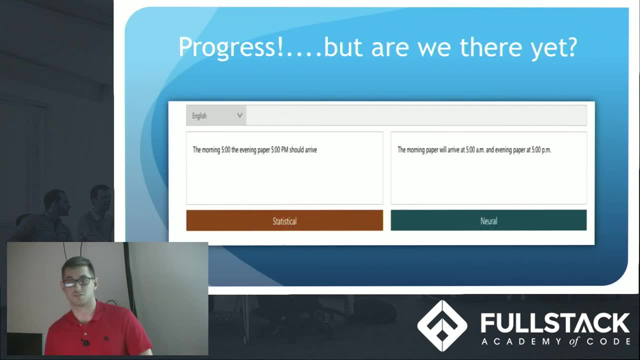 That doesn't sound great. And then you have the other translation: The morning paper will arrive at 5 am and evening paper at 5 pm. That seems like a lot more of a proper translation To the left is our statistical old model. 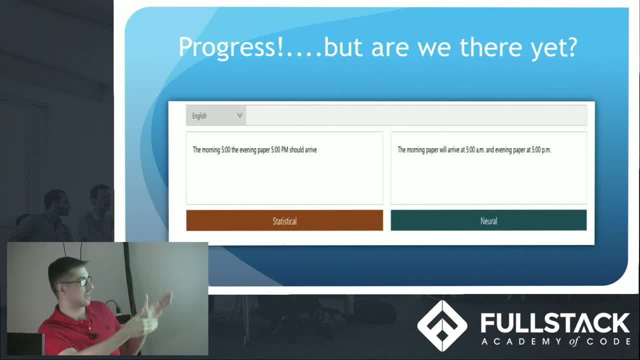 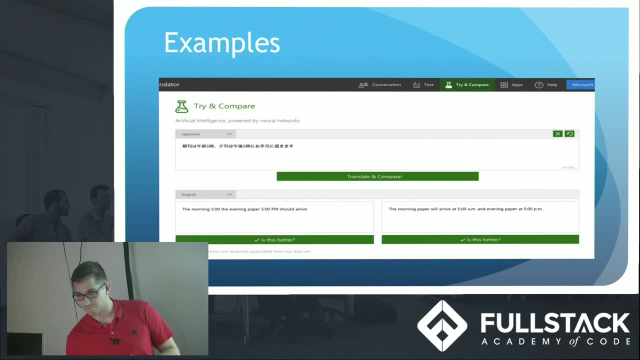 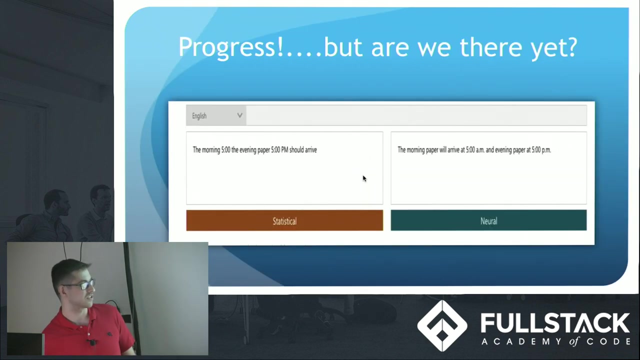 You can see almost how it's word by word in that model, how it was. Let me show you with my pointer here. So the morning 5, evening 5 will arrive, And it's broken down word by word. This neural translation just sounds more natural. 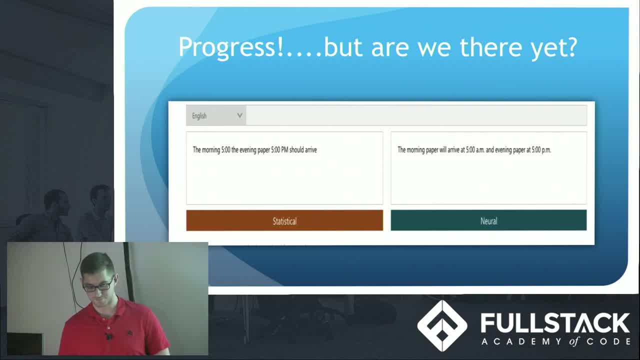 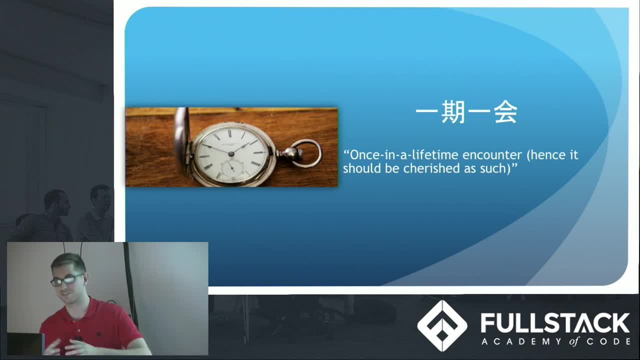 or, more appropriate, when speaking to someone else. Quick Japanese lesson for you guys. One of my favorite phrases is this word is this phrase called ichigo ichie, And it's not always easy to translate to English, but using this Japanese English dictionary, 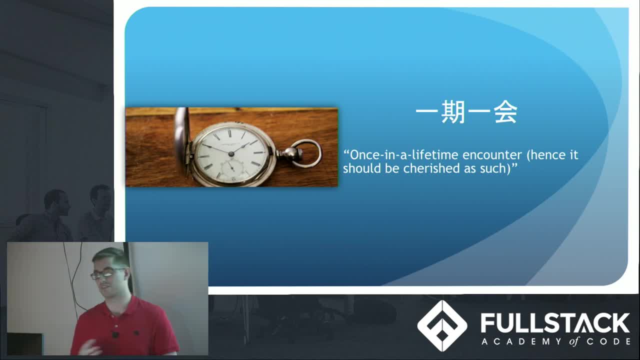 that I use online a lot. it's translated as a once in a lifetime encounter And hence it should be cherished as such. So as I was doing my research on NMT and seeing the progress, I was like, wow, I want to see what Google came up with for this. 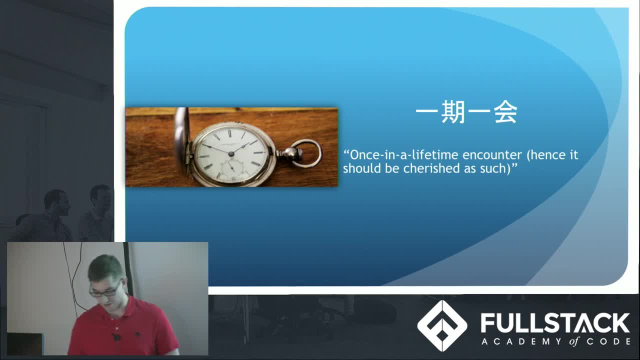 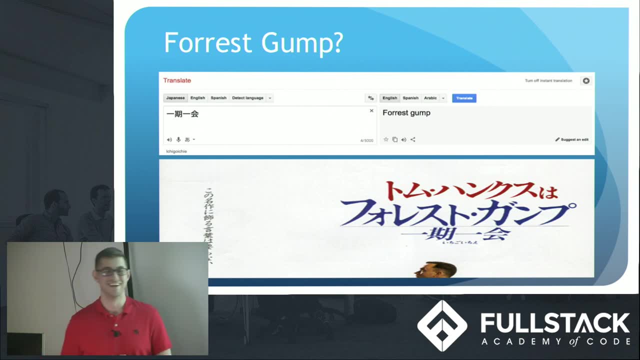 I want to see the difference And I was really surprised- and shocked actually- when I got Forrest Gump as the answer. I had no idea what was happening and was very confused until I dug a little deeper and found out that this is actually. this is also the subtitle to the Japanese version of Forrest Gump. 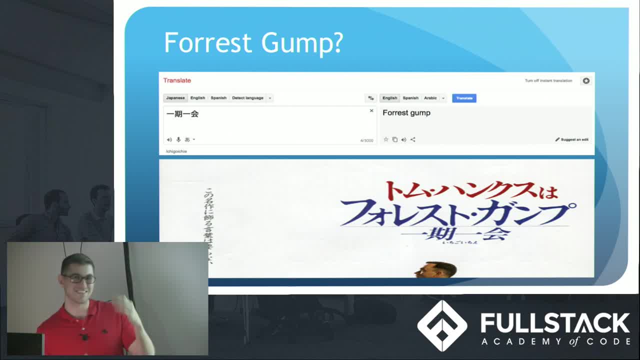 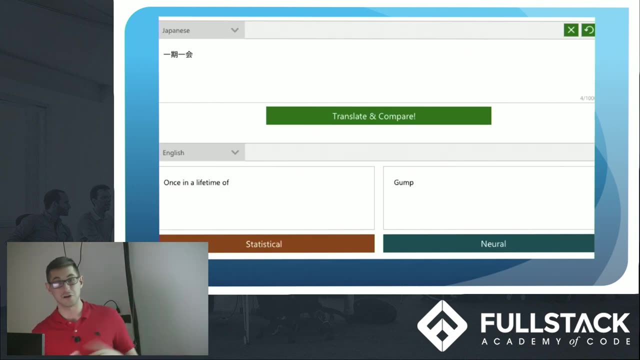 So, as it was going through the neural network, it probably saw this more than it saw that more difficult translation. And another interesting thing about it was when I put this through Microsoft Translate, the statistical model was actually closer. As you can see, one is Gump and the other is once in a lifetime. 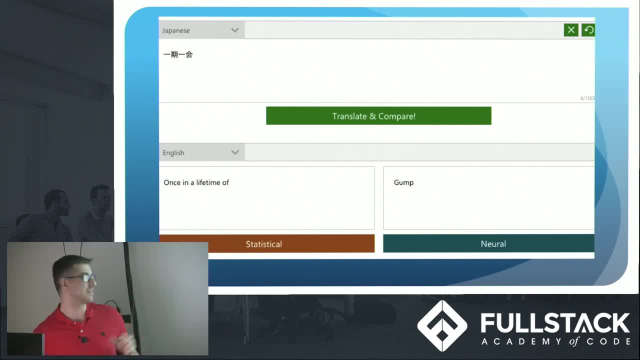 So it's still difficult And maybe there are times when we should be using, we should be going back to that statistical model, But the neural model has made huge progress And that's what I want to conclude with. Neural machine translation is really important.